50. 같습니다 qualité and all property of anytime. Our second example is the quarter number and the first number is the second. Now for L Şu, we write like this: Moron i haka hai, Hai hai. Are you reading this? 정부 ji ki mussahak lesti hai scenist, ai live it tu叫. 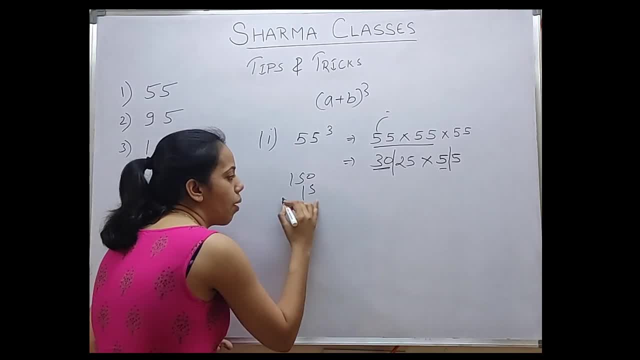 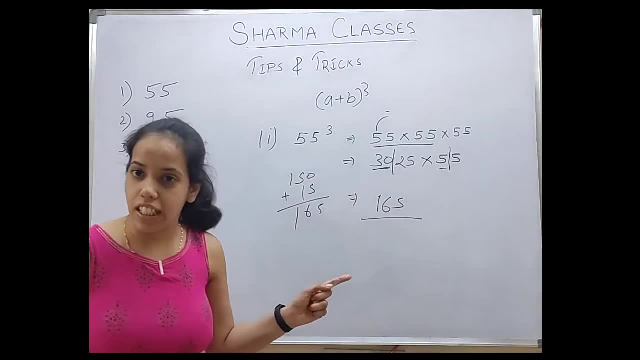 What is the half of 30? 30 ka, half 50. And in this number, half of 30.. 5, 5, 5, 1, 6,, 1, 65.. From here we get our first 3 digits. Yes, student, This is our. this is the 1, 65,, our first 3 digits of answer. 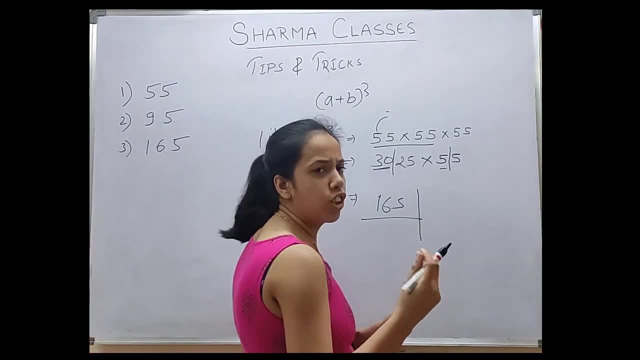 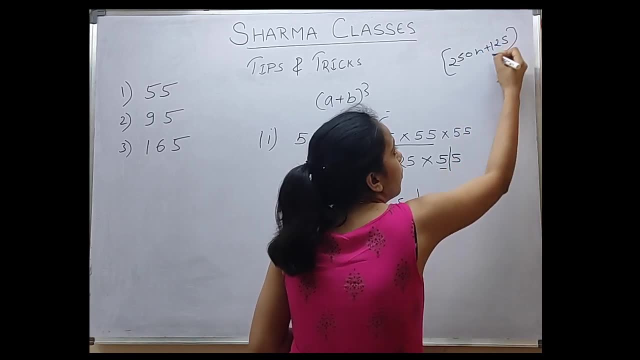 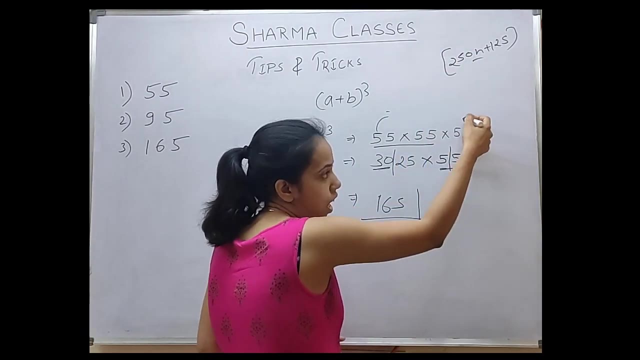 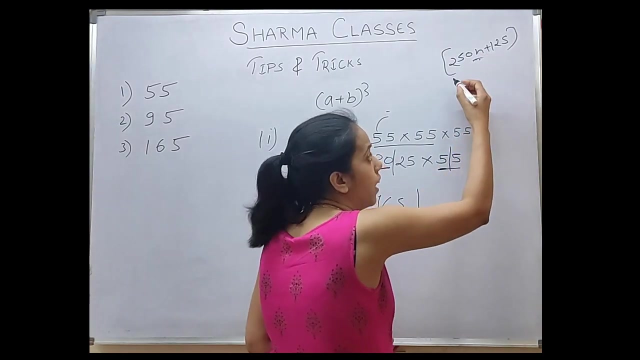 Now for next what we have to do. There is a small formula which you have to remember. Formula is 250 and plus 125.. Now, question is: what is our n? Okay, So what is n When we divided our number, whose cube we are taking out, into two portions, then the remaining part of it, the first remaining part, that is our n, That means 250 into 5 plus 125. 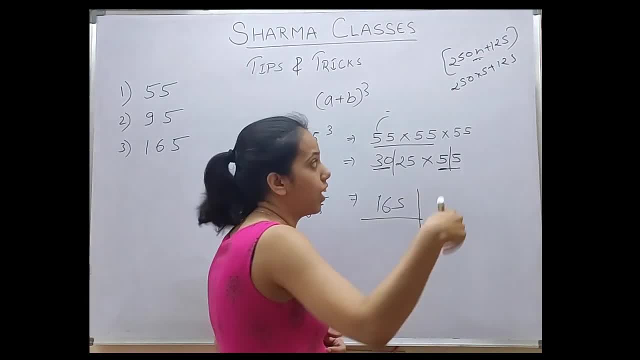 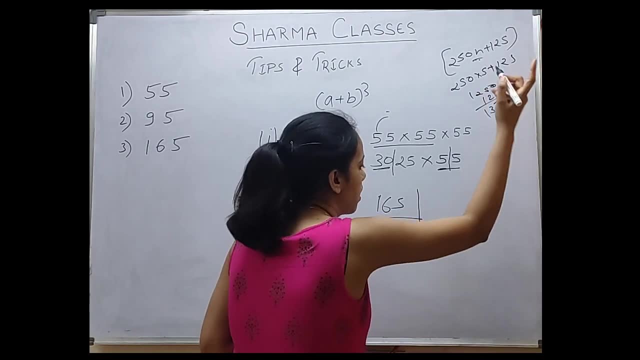 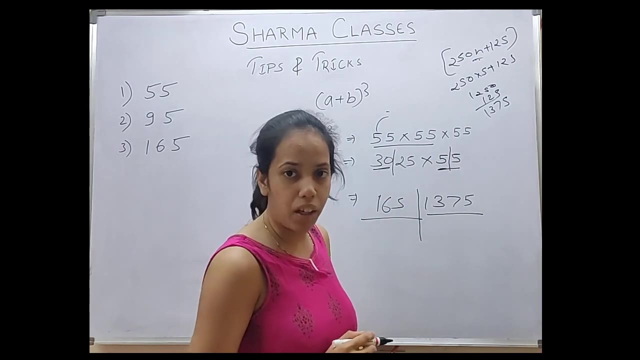 255 is what 255.. 125. Correct 125, means 1250 plus 125.. 5, 5, 2, 7, 2 or 1, 3 and 1, 3, 7, 5.. Correct, This is our last 4 digits. But because we are finding the cube of any number, that means we only take the last 3 digits from here. 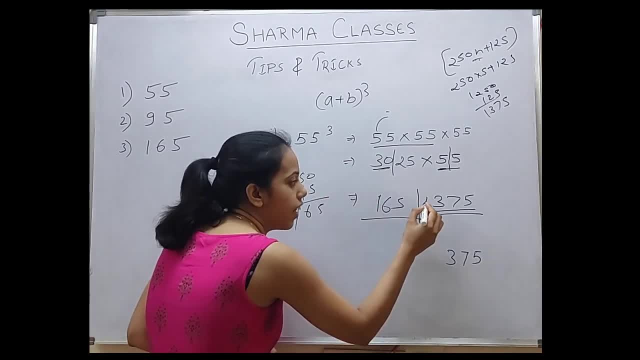 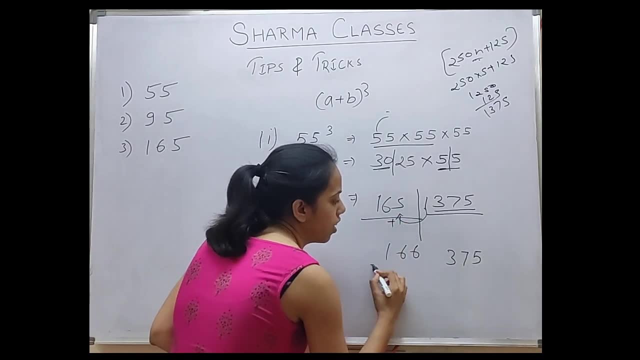 Our last 3 digits is 375.. And this one is carry forward from okay. So for 1, yeah, yeah, 1, I do a 5 or 1, 6,, 1, 6, 6, 1.. 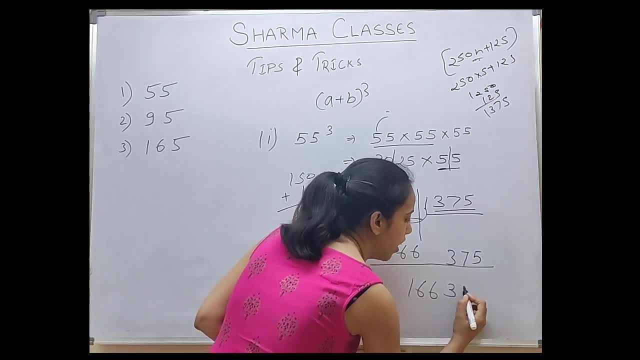 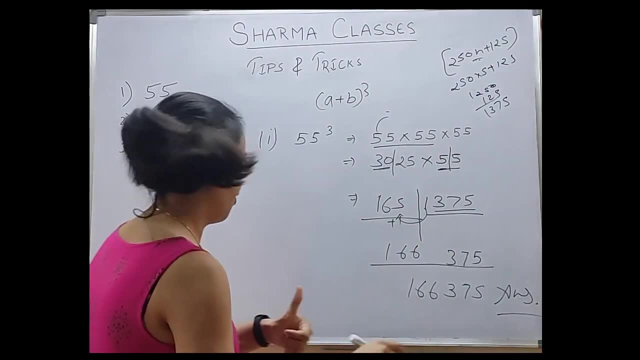 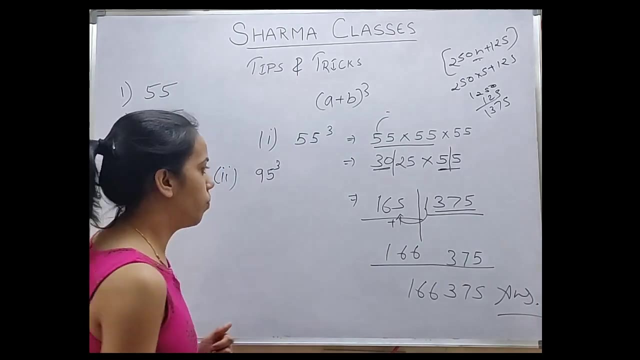 6, 3, 6, 3, 75.. Yes, yes, student. 1, 3, 1, 6, 3, 75 is 5 is our answer, Okay. Second example: We take one more example. Our second example is cube of 95.. 95's cube: 95 multiplied by 95, multiplied by 95. Okay. 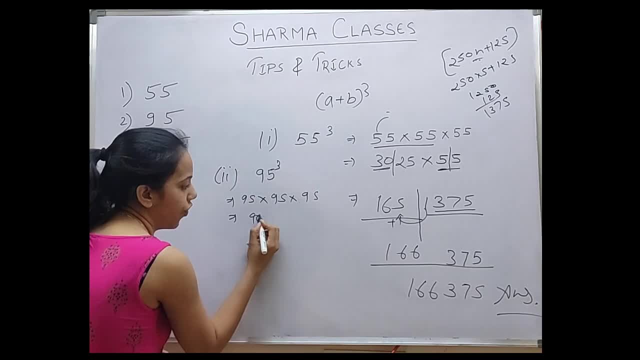 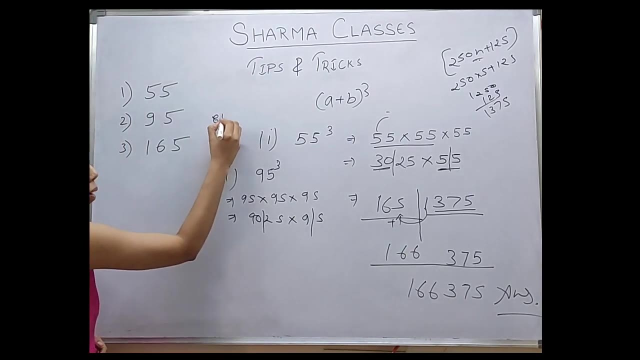 95's square. What is the 95's square? 9025.. Right Into 95.. Okay, Divided the number into two parts: 90, 90 and 90.. 90 into 9.. 90 into 9, 810.. 810 plus 90's half 45. 855.. Our first 3 digits is 855.. Correct, Now digit. For next digit, what do we have to do? 250 into n plus 125.. N's value from here is 9.. 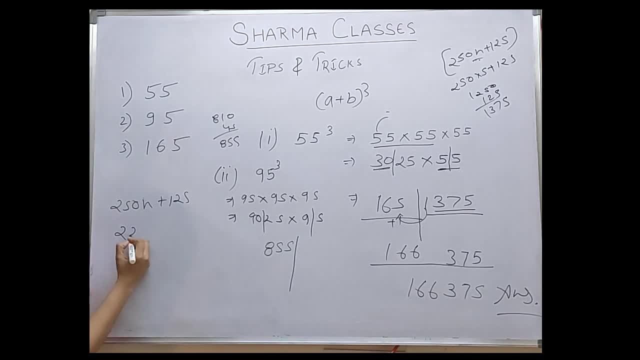 25 into 9.. 25 into 9.. 225 at 0 plus 125.. 5's, 5.. 5 or 2, 7. 2 or 1, 3.. 2's, 2. 2375.. 2375.. Next step: just send 2 here. You don't want 2, right, Send it. Send it. What is 5 plus 2? 7.. The rest of the digits will remain the same: 375.. This is our answer, students. 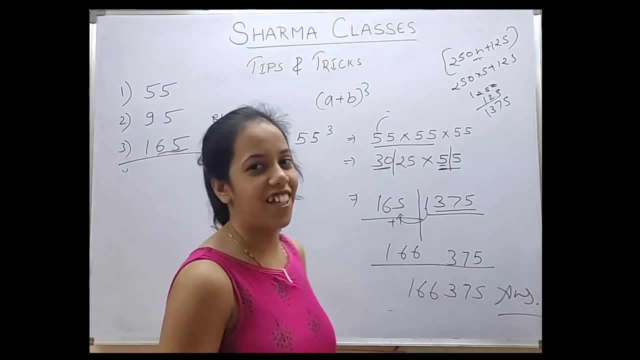 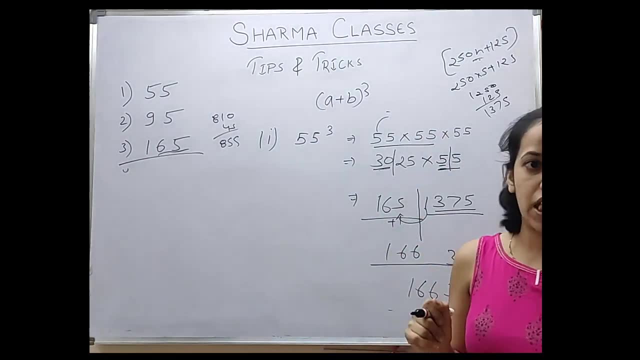 Okay, So did you enjoy it? So did we understand the above example. Now we will start the 3rd one. Now you are thinking that 2 digits is easy than 3 digits will make the calculation increase. моh right, it will increase, But it will be a little increase. 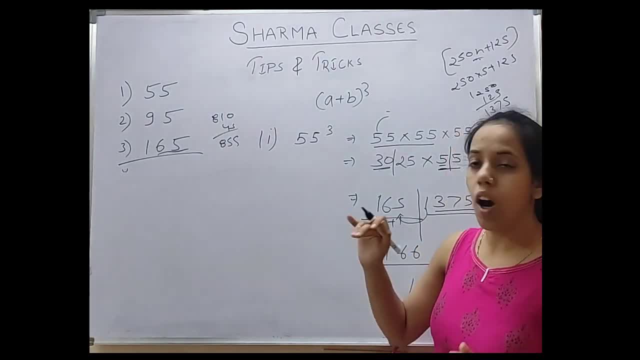 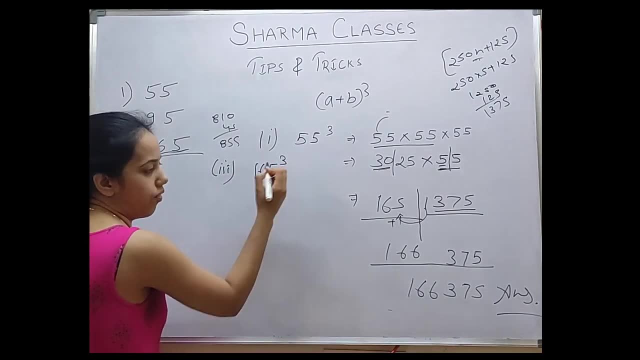 Because the calculation is easier from the especie lead inqu мираeere. Therefore, the 3th example will be about 3 digits. Our 3rd example is cube of 165, right, Find the cube of 165. 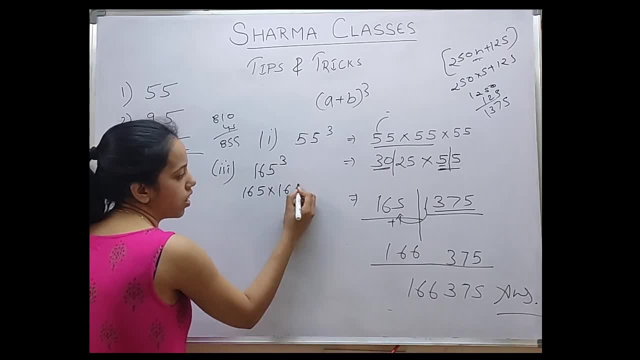 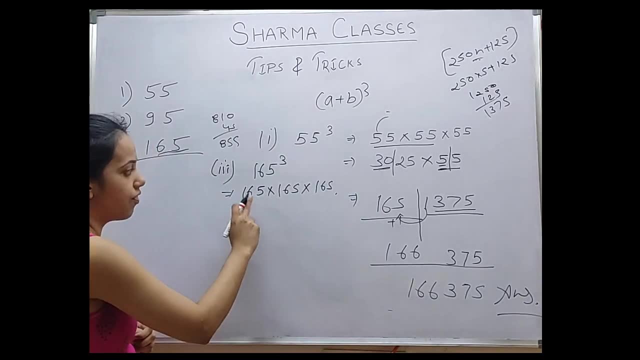 ¨What we do college. The first step is 165 multiplied by 165.. ¨What we ¨Не is 165 x 165 x 165.. From here, what will we do? What will we get out of 165? Square. 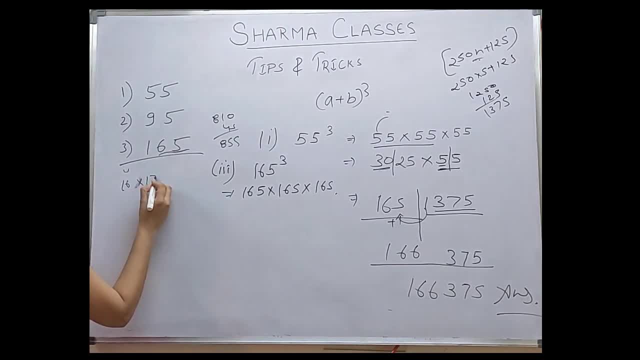 So to multiply 165, 16 x 17.. 16 x 17,, that means 7 x 6, is 42,, 2 carry over 4, 7 x 7 over 4,, 11.. And 16 x 16, 2,, 2, 6 over 1, 7, or 2, 2,, 7, 2 and 2, 5.. Last digits are same. 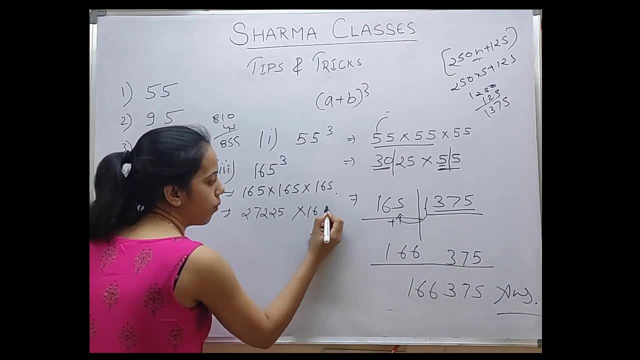 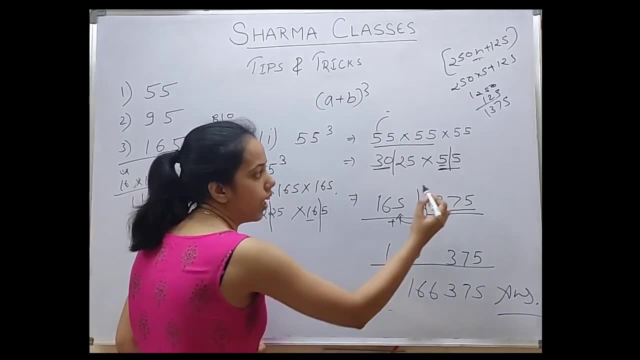 in 25 square. Okay, now multiply by 165.. Next step: what is the next step? Divide number 2 parts. Divide over here. here 2 digits are there. here 1 digit is there. Because here 2 digits are there, we have divided in 2 portions, We have to cut the unit digit and 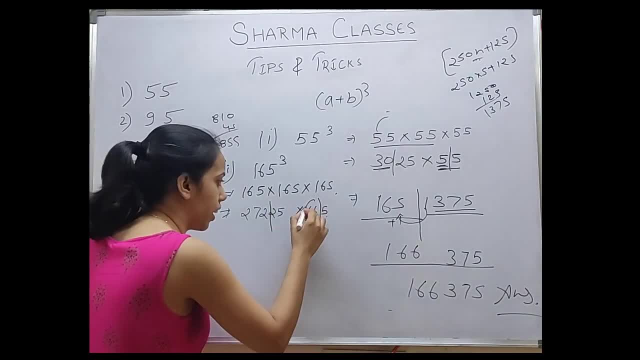 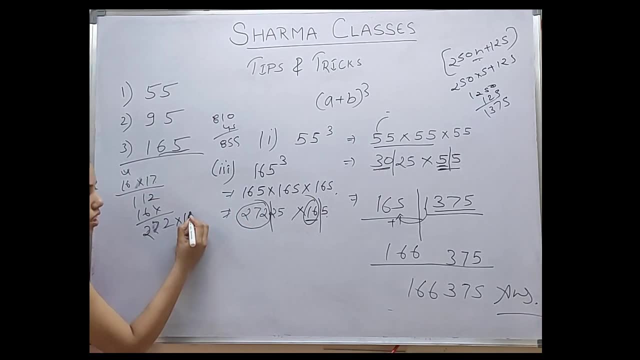 whatever number is remaining, we have to divide it. So we have to divide the unit and take the whole number. Yeah, correct, Now from here, 16 x 272.. Now, what will we do? We will multiply 272 with what 16.. Do it: 6 x 2 is 12,. 2 carry over 1,. 6 x 7 is. 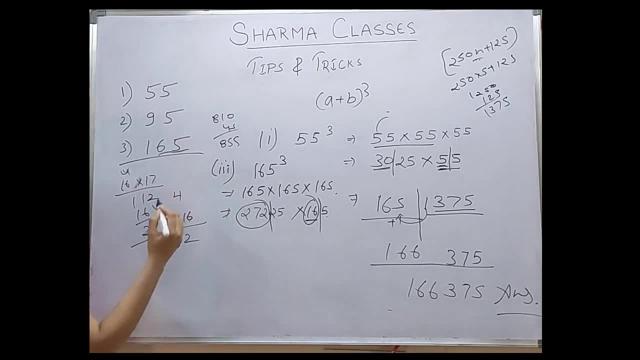 42 and 1 is 43.. 4 carry over 6 x 2 is 12 and 4.. Yes, 16.. Now 272.. 2 x 2 is 2, 3 x 2 is 5, 6 x 7 is 6 and 7 is 13.. 2 over 1, 3 over 1, 4.. Now, what will we do? We will multiply. 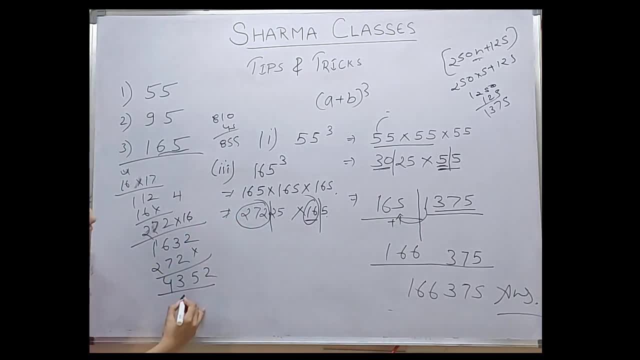 the same 272 half. If we do half of 272, then it will come 1, 3, 6.. Right Now, add 6 over 2, 8,, 5 over 3, 8, 3 over 1, 4, 4.. Okay, our first 4 digits we have got from here. Yes. 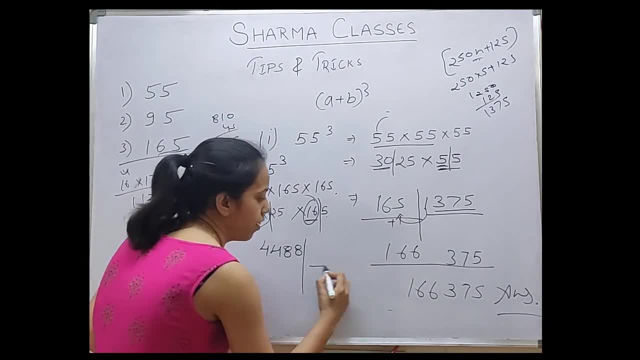 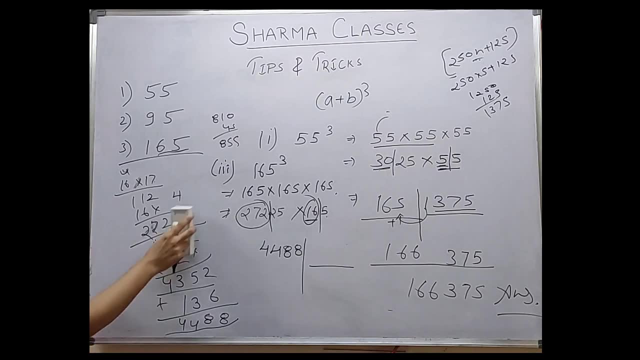 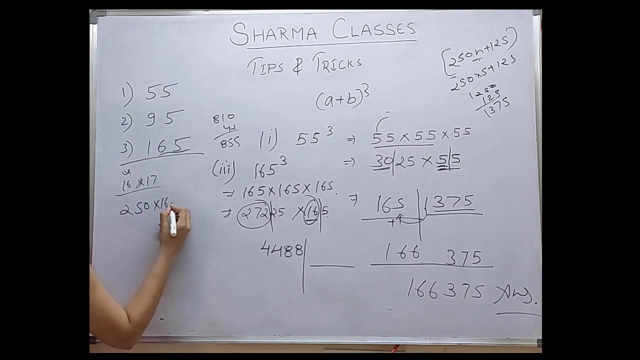 these are our first 4 digits. Now what to do? Same Next digit: Find last digit. Find last digit For last digit. what to do? Apply formula: What is the formula? 250 x n plus 125.. 250 x 16 plus 125.. Now what to do? 250 x 8, that is how much, How much. 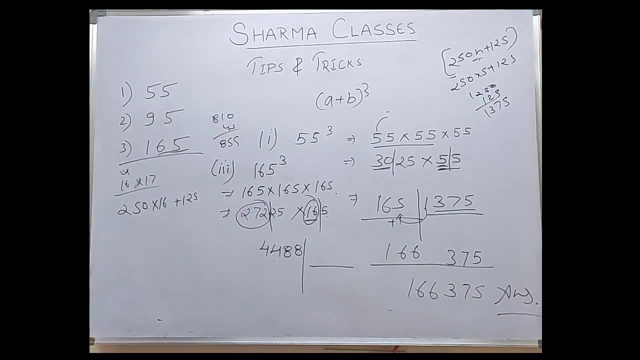 does it make 4000.. Am I correct? No, no, How? I have multiplied it by 16.. Atleast, check 25, 250 x it. What does it make? Multiply it by 16,, then 4,000.. If we multiply by 8,, 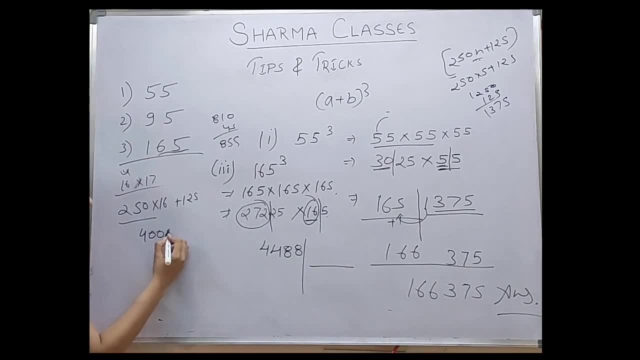 how much will it come? 2000.. Correct, no. Multiply it by 16, then 4,000 will come, If We have to add this digit in 4000.. That's it: 4, 1,, 2, 5.. 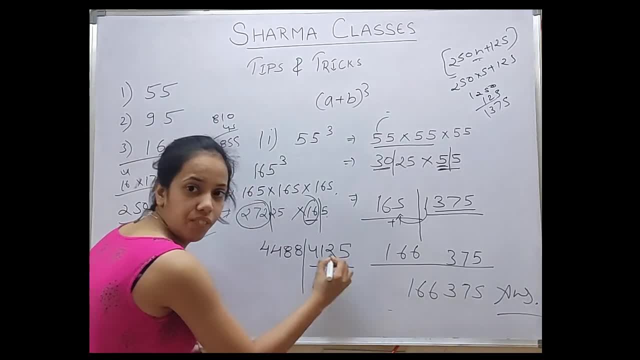 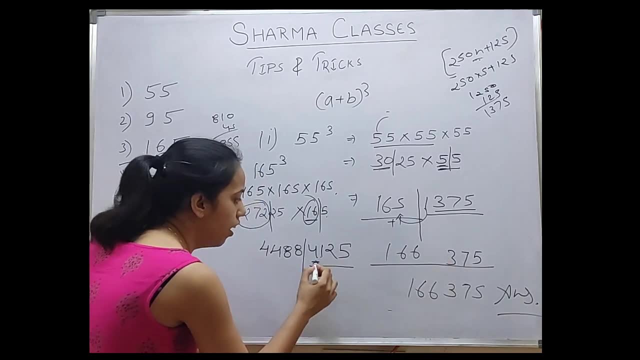 Yes, Last 4 digits: 4, 1,, 2, 5.. Correct Now what we have to do. This last number, 3 digits. We have to find the cube Leaving 3 digits. We have to send it here. 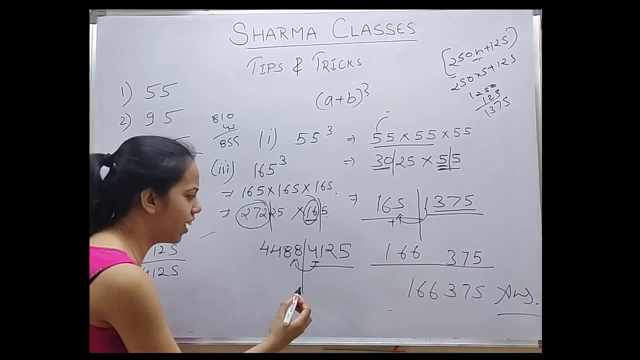 We don't have to keep 4.. We have to remove 4 from the house. We have to add 4 in 8.. 8 and 4 is 12.. Do you want to carry over 1?? 8 and 1 is 9..